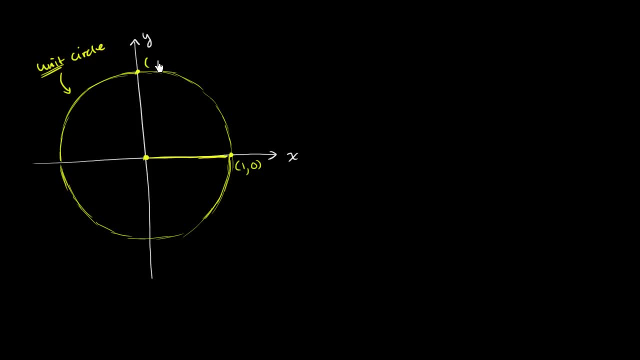 Well, we've gone 1 above the origin, but we haven't moved to the left or the right. So our x value is 0, our y value is 1.. What about back here? Well, here our x value is negative, 1.. 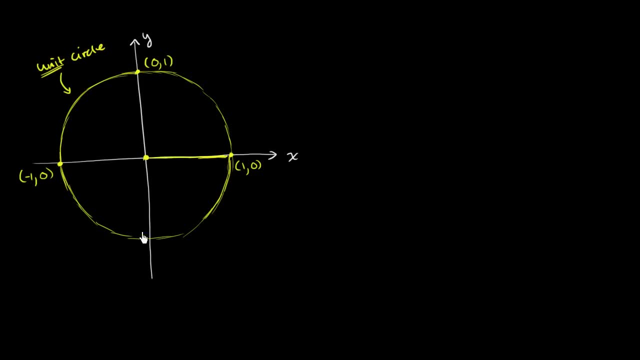 We've moved 1 to the left and we haven't moved up or down. So our y value is 0.. And what about down here? Well, we've gone a unit down Or 1 below the origin, but we haven't. 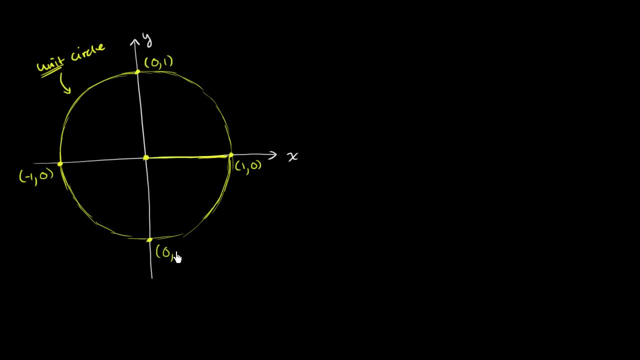 moved in the xy direction. So our x is 0, and our y is negative 1.. Now, with that, out of the way I'm going to draw an angle And the way I'm going to draw this angle, I'm going to define a convention for positive angles. 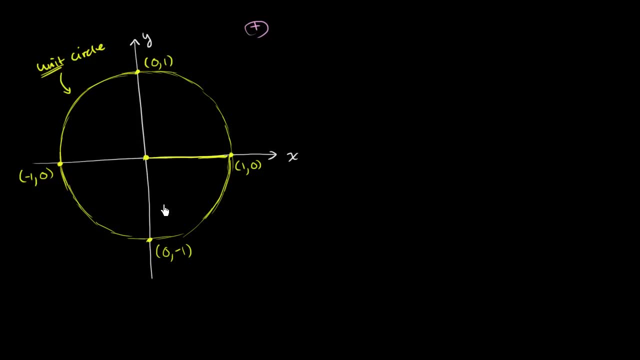 I'm going to say a positive angle. Well, the initial side of an angle we're always going to do along the positive x-axis. So this is the starting side of the angle, the initial side of an angle, And then to draw an angle, a positive angle, 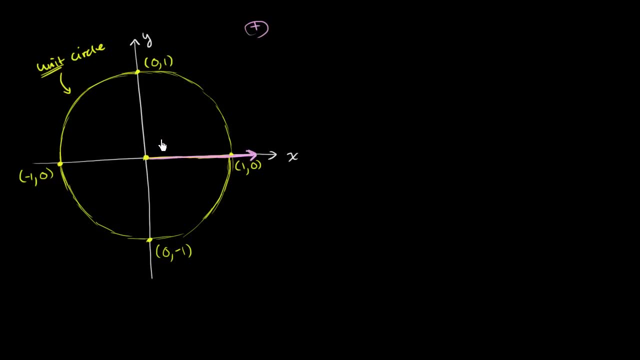 the terminal side, we're going to move in a counterclockwise direction. So positive angle means we're going counterclockwise, And this is just the convention I'm going to use, And it's also the convention that is typically used. 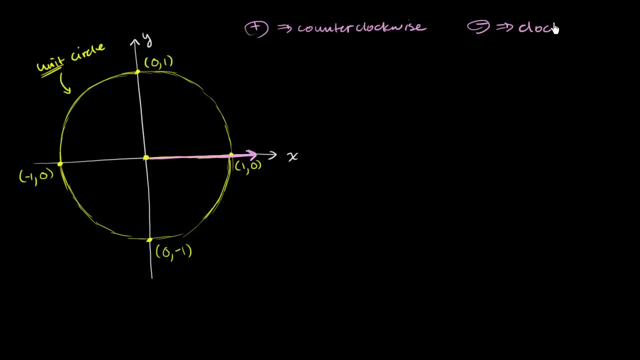 And so you can imagine a negative angle would move in a clockwise direction. So let me draw a positive angle. So a positive angle might look like this, It might look something like this: This is the initial side, And then from that I go in a counterclockwise direction. 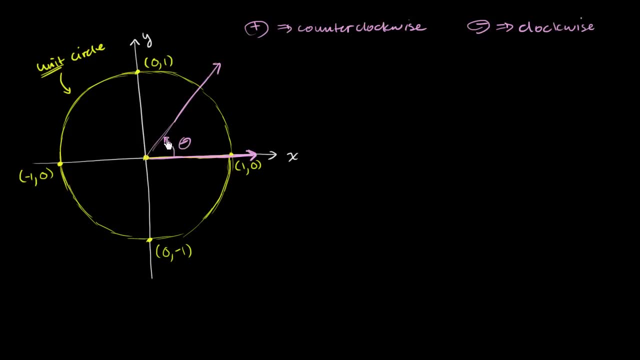 until I measure out the angle And then this is the terminal side. So this is a positive angle, theta, And what I want to do is think about this point of intersection between the terminal side of this angle and my unit circle. And let's just say it has the coordinates a, comma b, 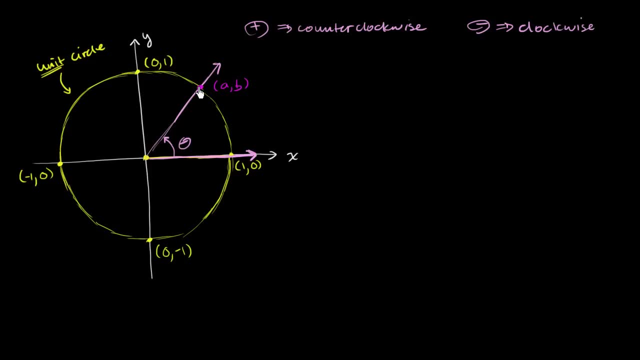 The x value where it intersects is a, The y value where it intersects is b. So I'm going to draw a positive angle. The x value where it intersects is b, And I'm also the whole point of what I'm doing here. 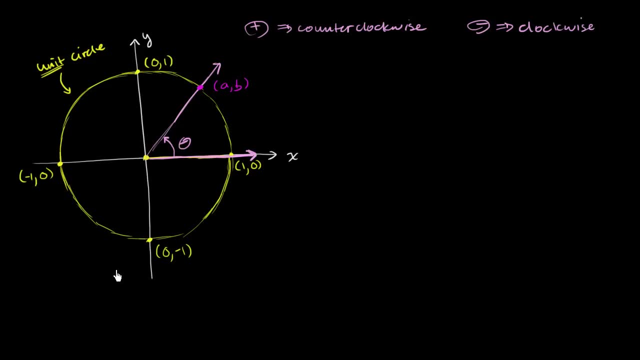 is. I'm going to see how this unit circle might be able to help us extend our traditional definitions of trig functions, And so what I want to do is I want to make this theta part of a right triangle. So, to make it part of a right triangle. 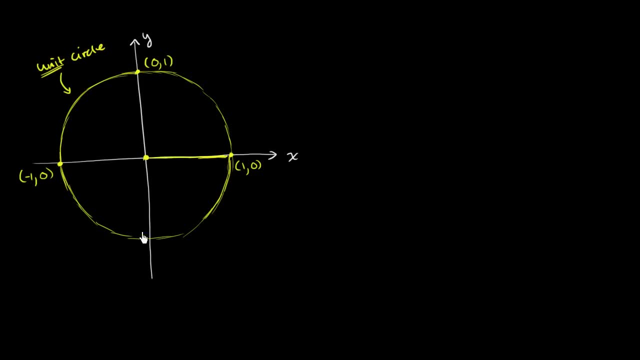 We've moved 1 to the left and we haven't moved up or down. So our y value is 0.. And what about down here? Well, we've gone a unit down Or 1 below the origin, but we haven't. 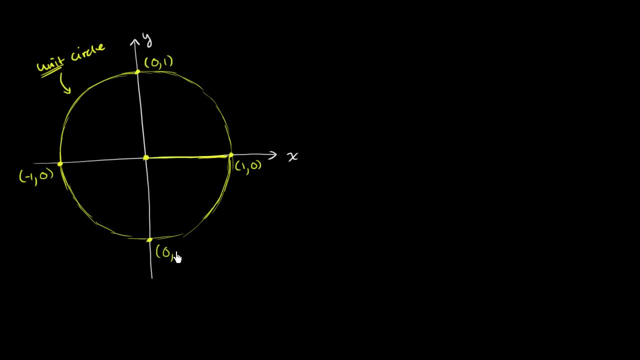 moved in the xy direction. So our x is 0, and our y is negative 1.. Now, with that, out of the way I'm going to draw an angle And the way I'm going to draw this angle, I'm going to define a convention for positive angles. 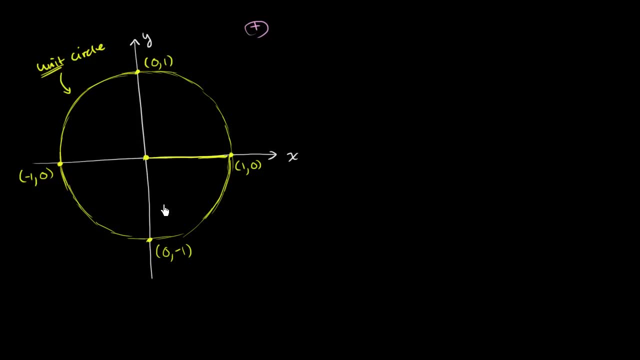 I'm going to say a positive angle. Well, the initial side of an angle we're always going to do along the positive x-axis. So this is the starting side of the angle, the initial side of an angle, And then to draw an angle, a positive angle, 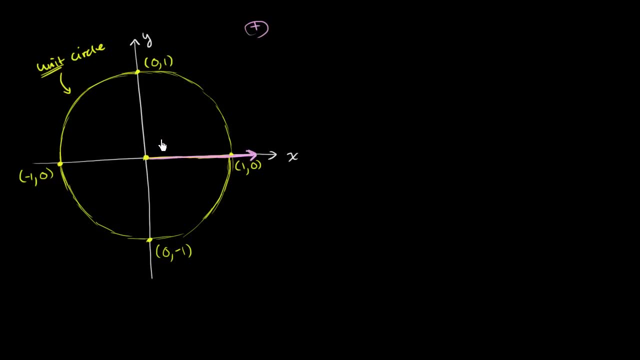 the terminal side, we're going to move in a counterclockwise direction. So positive angle means we're going counterclockwise, And this is just the convention I'm going to use, And it's also the convention that is typically used. 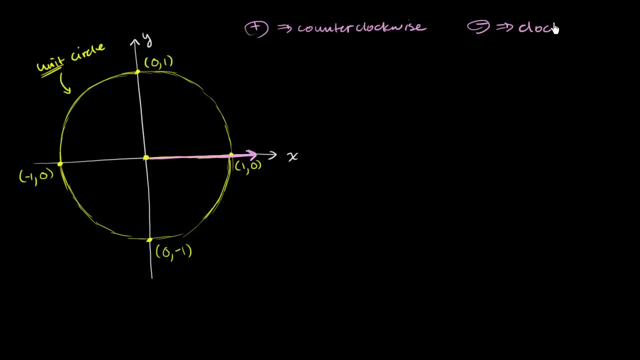 And so you can imagine a negative angle would move in a clockwise direction. So let me draw a positive angle. So a positive angle might look like this, It might look something like this: This is the initial side, And then from that I go in a counterclockwise direction. 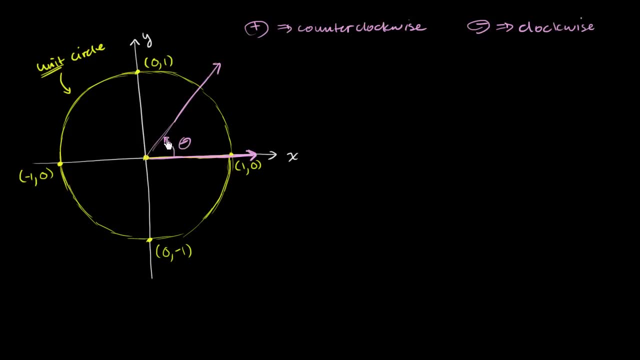 until I measure out the angle And then this is the terminal side. So this is a positive angle, theta, And what I want to do is think about this point of intersection between the terminal side of this angle and my unit circle. And let's just say it has the coordinates a, comma b, 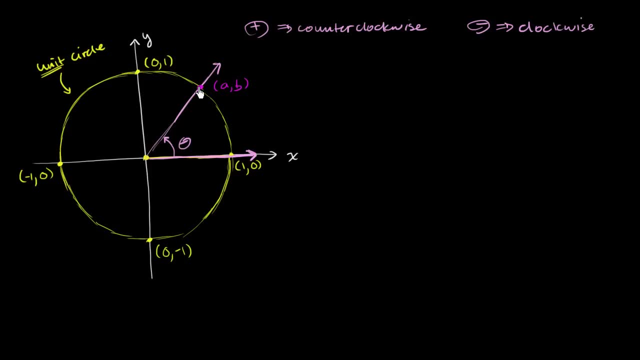 The x value where it intersects is a, The y value where it intersects is b. So I'm going to draw a positive angle. The x value where it intersects is b, And I'm also the whole point of what I'm doing here. 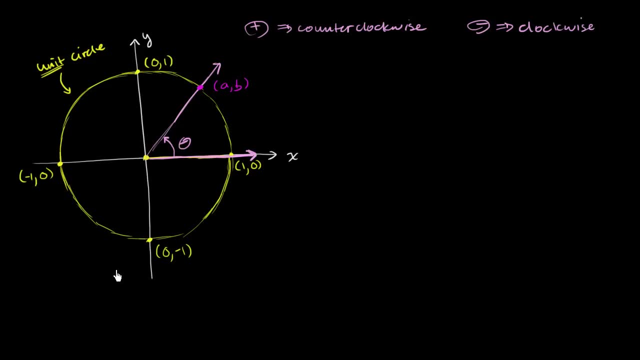 is. I'm going to see how this unit circle might be able to help us extend our traditional definitions of trig functions, And so what I want to do is I want to make this theta part of a right triangle. So, to make it part of a right triangle. 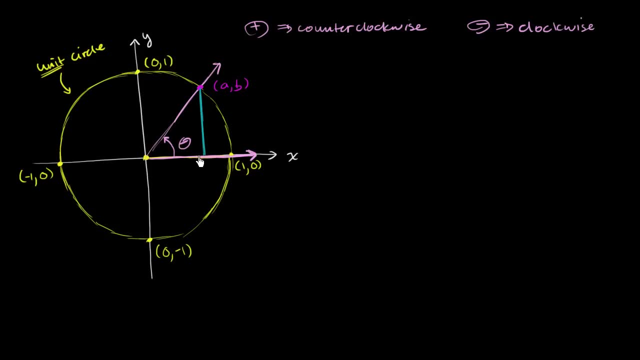 let me drop an altitude right over here And let me make it clear that this is a 90 degree angle. So this theta is part of this, This right triangle. So let's see what we can figure out about the sides of this right triangle. 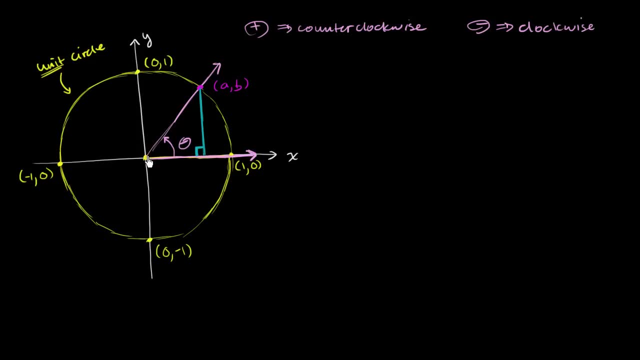 So the first question I have to ask you is: what is the length of the hypotenuse? What is the length of the hypotenuse of this right triangle that I have just constructed? Well, this hypotenuse is just a radius of a unit circle. 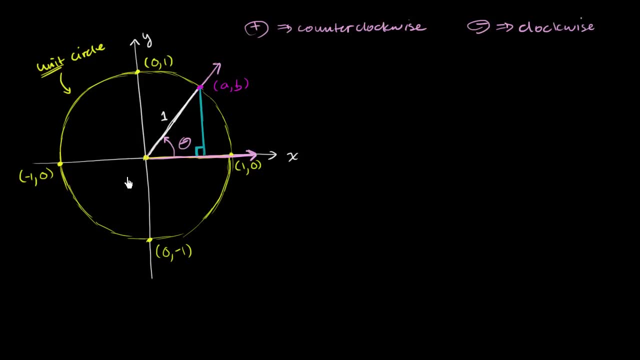 The unit circle has a radius of 1.. So the hypotenuse has length 1.. Now, what is the length of this? This blue side right over here, This blue side? You could view this as the opposite side to the angle. 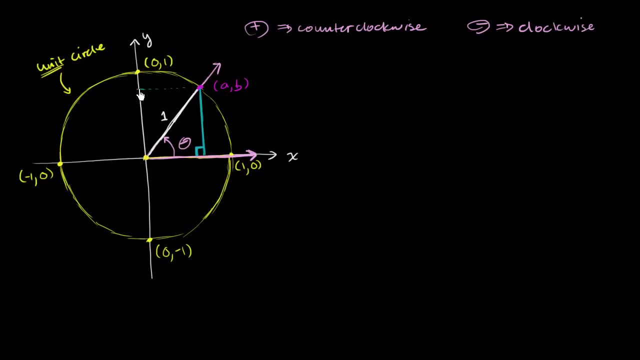 Well, this height is the exact same thing as the y-coordinate of this point of intersection. So this height right over here is going to be equal to b. The y-coordinate right over here is b. This height is equal to b. Now, exact same logic. 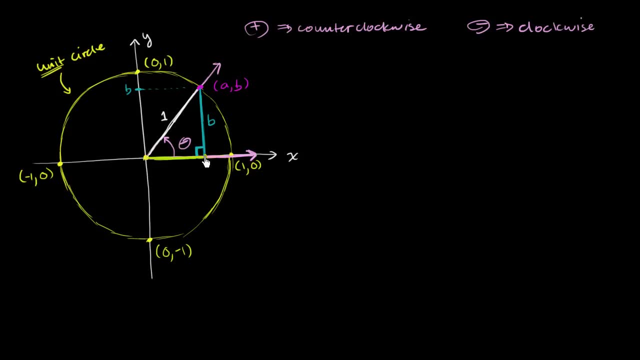 What is the length of this base going to be? The base, Just, of the right triangle. Well, this is going to be the x-coordinate of this point of intersection. If you were to drop this down, this is the point. x is equal to a. 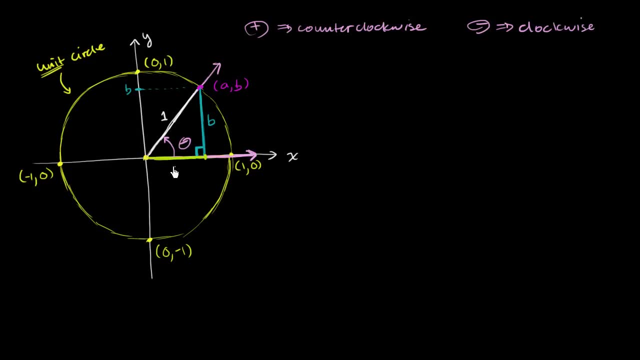 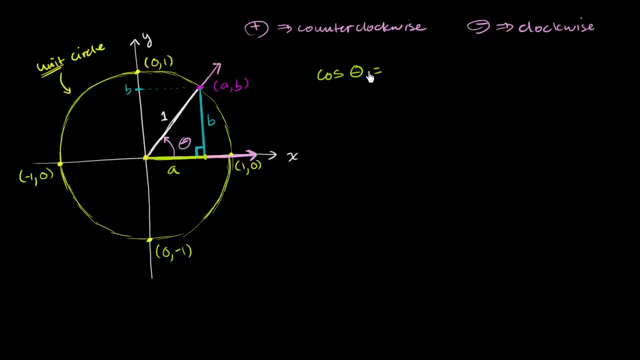 What is the cosine of my angle going to be in terms of a's and b's and any other numbers that might show up? Well, to think about that, we just need our SOHCAHTOA definition. That's the only one we have now. 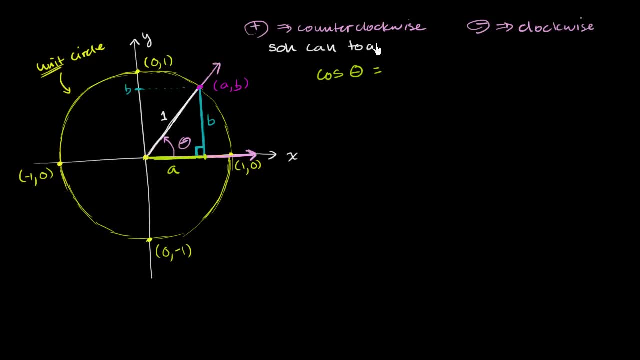 We are actually in the process of extending it. SOHCAHTOA definition of trig functions, And the ca part is what helps us with cosine. It tells us that the cosine of an angle is equal to the length of the adjacent side over the hypotenuse. 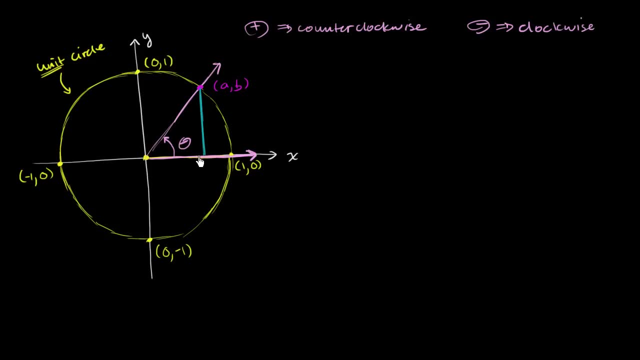 let me drop an altitude right over here And let me make it clear that this is a 90 degree angle. So this theta is part of this, This right triangle. So let's see what we can figure out about the sides of this right triangle. 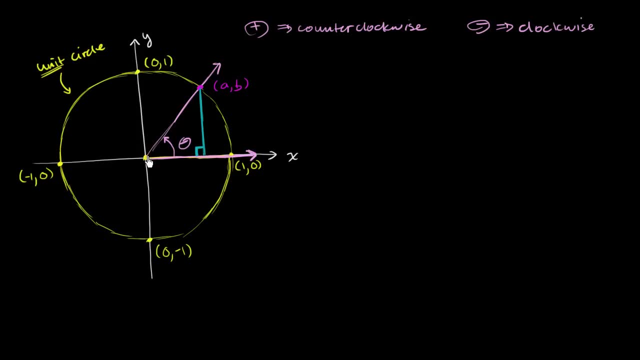 So the first question I have to ask you is: what is the length of the hypotenuse? What is the length of the hypotenuse of this right triangle that I have just constructed? Well, this hypotenuse is just a radius of a unit circle. 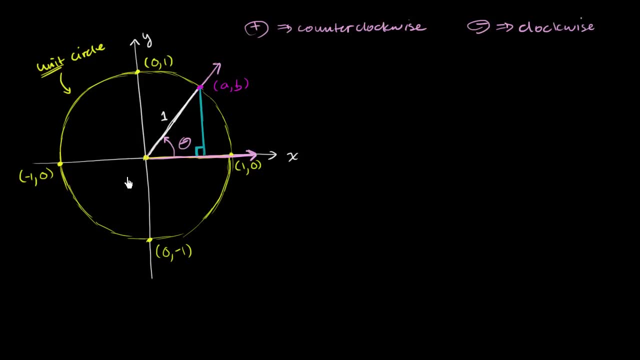 The unit circle has a radius of 1.. So the hypotenuse has length 1.. Now, what is the length of this? This blue side right over here, This blue side? You could view this as the opposite side to the angle. 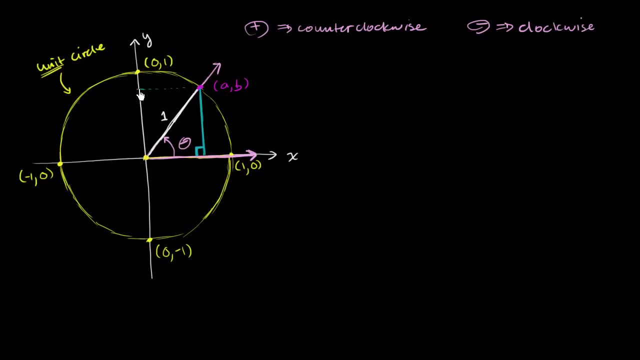 Well, this height is the exact same thing as the y-coordinate of this point of intersection. So this height right over here is going to be equal to b. The y-coordinate right over here is b. This height is equal to b. Now, exact same logic. 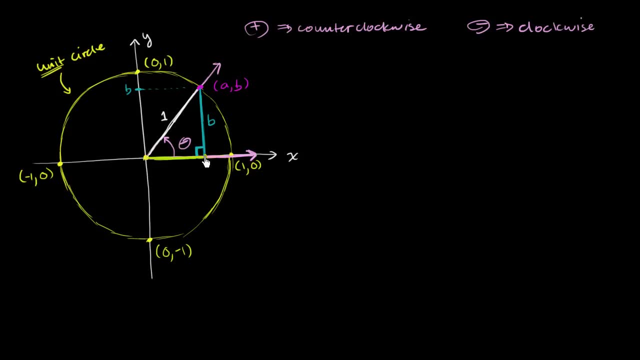 What is the length of this base going to be? The base, Just, of the right triangle. Well, this is going to be the x-coordinate of this point of intersection. If you were to drop this down, this is the point. x is equal to a. 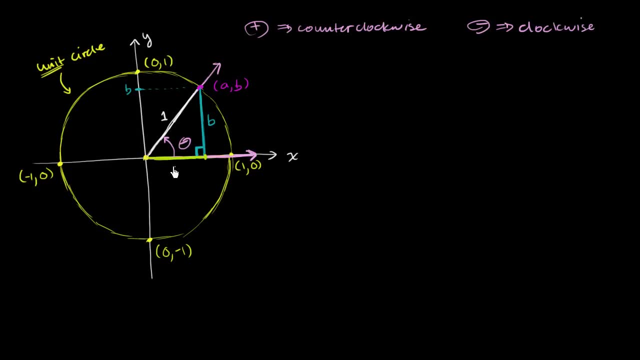 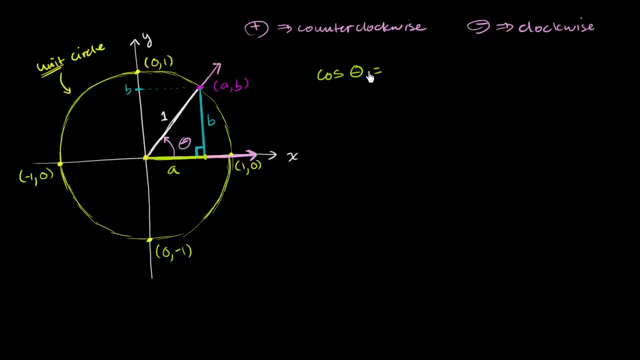 What is the cosine of my angle going to be in terms of a's and b's and any other numbers that might show up? Well, to think about that, we just need our SOHCAHTOA definition. That's the only one we have now. 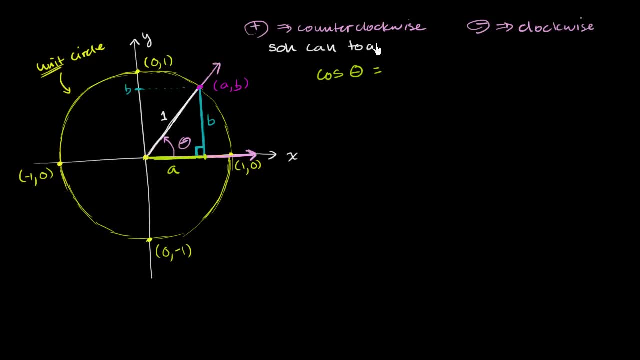 We are actually in the process of extending it. SOHCAHTOA definition of trig functions, And the ca part is what helps us with cosine. It tells us that the cosine of an angle is equal to the length of the adjacent side over the hypotenuse. 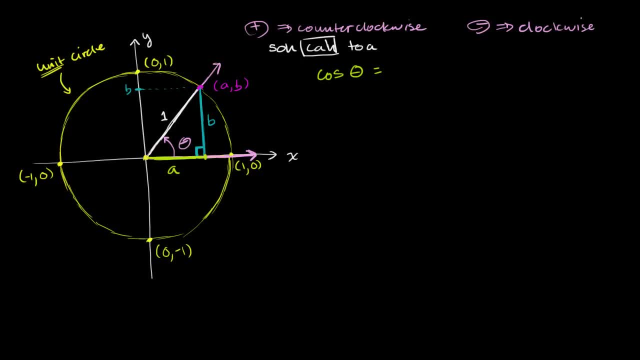 So what's this going to be? The length of the adjacent side. For this angle, the adjacent side has length a, So it's going to be equal to a over what's the length of the hypotenuse? Well, that's just 1.. 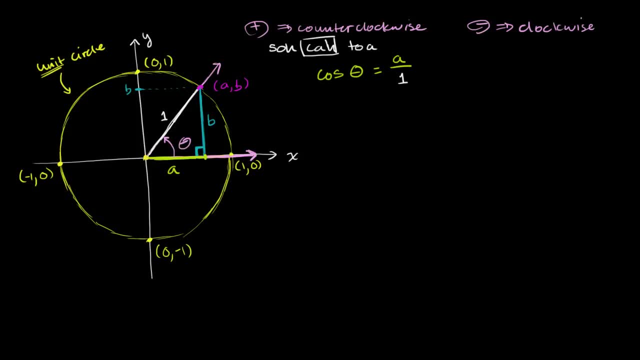 So the cosine of theta is just equal to a. Let me write this down again. So the cosine of theta is just equal to a. It's equal to the x-coordinate of where this terminal side of the angle intersected, the unit circle. Now let's think about the sine of theta. 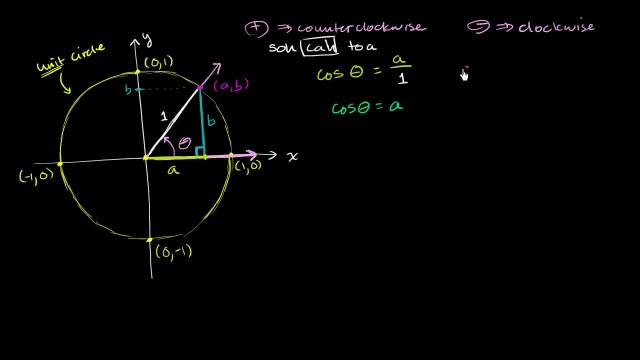 And I'm going to do it in orange. So what's the sine of theta going to be? Well, we just have to look at the SOH part of our SOHCAHTOA definition. It tells us that sine is opposite. over hypotenuse. 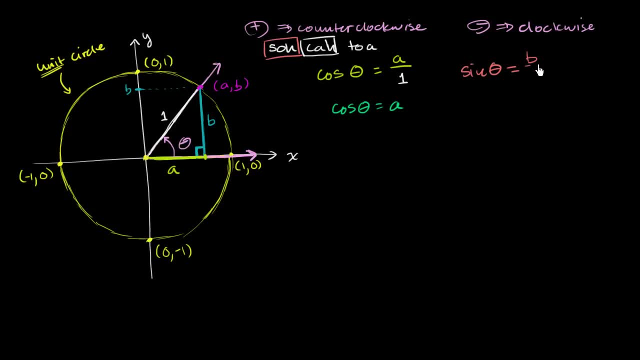 Well, the opposite side here has length b And the hypotenuse has length 1.. So our sine of theta is equal to b. So an interesting thing. This coordinate this point where our terminal side of our angle intersected the unit circle. 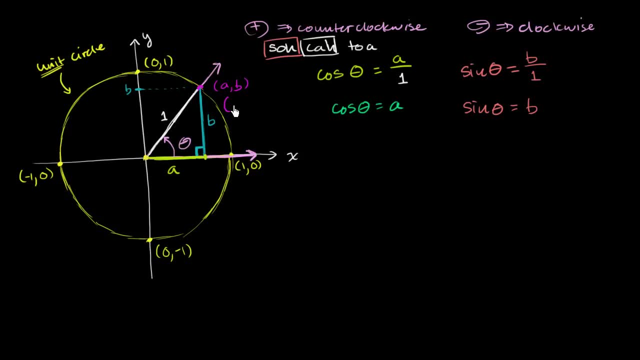 that point a- b. we could also view this as: a is the same thing as cosine of theta And b is the same thing as sine of theta. Well, that's interesting. That was just. we used our SOHCAHTOA definition. 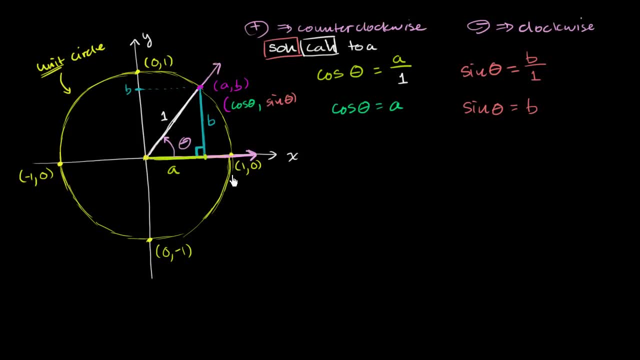 Now can we in some way use this to extend SOHCAHTOA, Because SOHCAHTOA Well a problem. It works out fine if our angle is greater than 0 degrees- if we're dealing with degrees- and if it's less than 90. 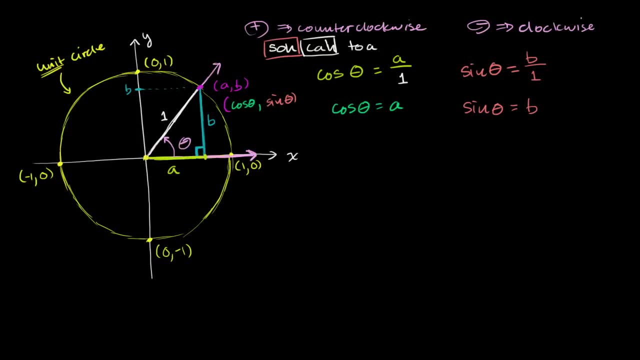 degrees. We can always make it part of a right triangle, But SOHCAHTOA starts to break down as our angle is either 0, or maybe even becomes negative, or as our angle is 90 degrees or more. You can't have a right triangle with two 90 degree angles in it. 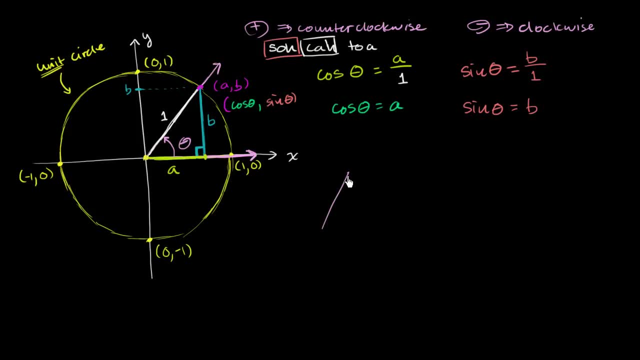 It starts to break down. Let me make this clear. So sure this is a right triangle, so the angle is pretty large. I can make the angle even larger and still have a right triangle even larger, But I can never get quite to 90 degrees. 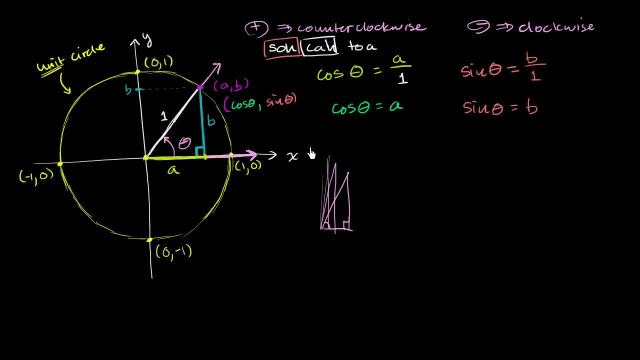 At 90 degrees it's not clear that I have a right triangle anymore. It all seems to break down, and especially the case what happens when I go beyond 90 degrees. So let's see if we can use what we set up here. 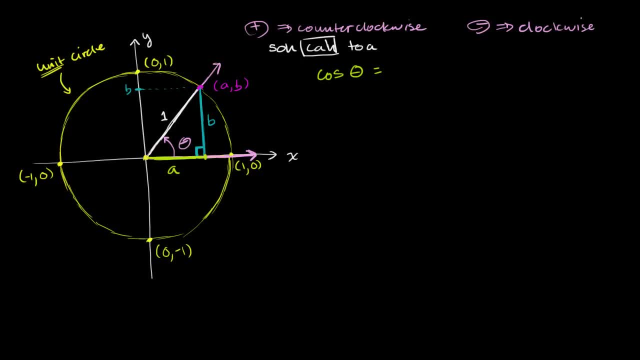 So what's this going to be? The length of the adjacent side. For this angle, the adjacent side has length a, So it's going to be equal to a over what's the length of the hypotenuse? Well, that's just 1.. 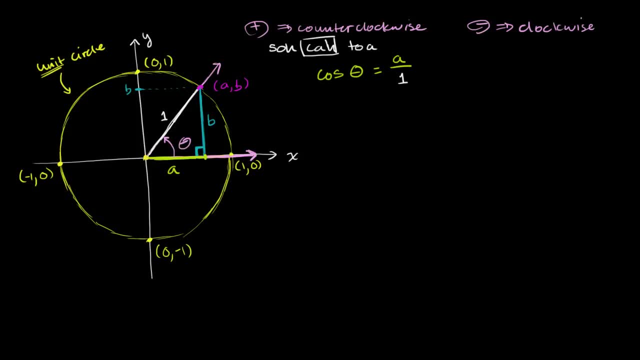 So the cosine of theta is just equal to a. Let me write this down again. So the cosine of theta is just equal to a. It's equal to the x-coordinate of where this terminal side of the angle intersected, the unit circle. Now let's think about the sine of theta. 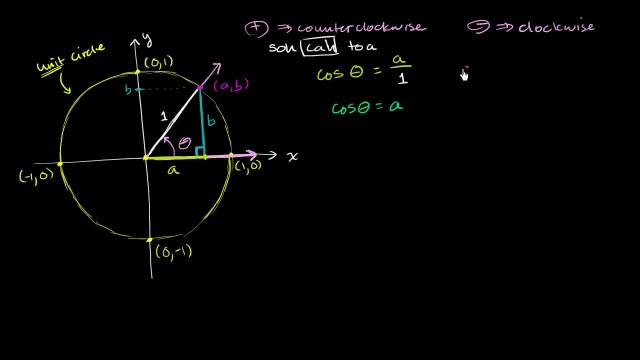 And I'm going to do it in orange. So what's the sine of theta going to be? Well, we just have to look at the SOH part of our SOHCAHTOA definition. It tells us that sine is opposite. over hypotenuse. 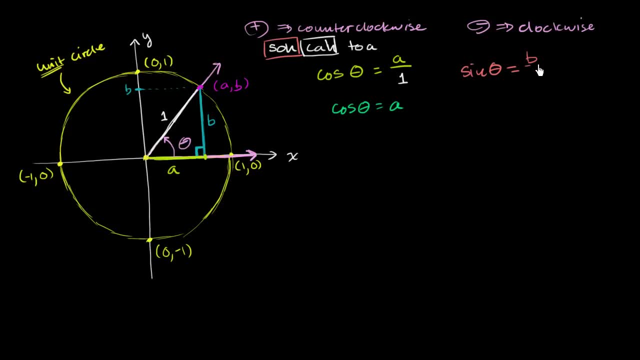 Well, the opposite side here has length b And the hypotenuse has length 1.. So our sine of theta is equal to b. So an interesting thing. this coordinate this point where our terminal side of our angle intersected, the unit circle, that point a- b. 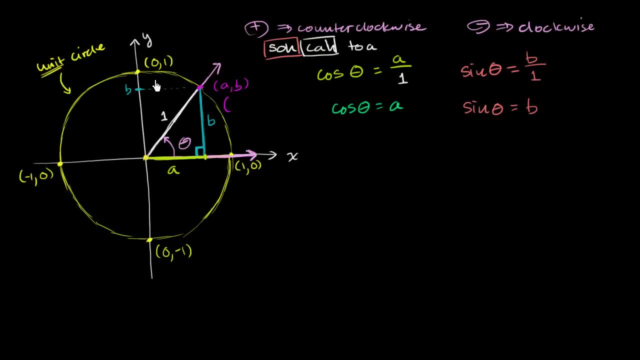 we could also view this as: a is the same thing as cosine of theta and b is the same thing as sine of theta. Well, that's interesting. That was just. we just use our SOHCAHTOA definition. Now can we in some way use this to extend SOHCAHTOA? 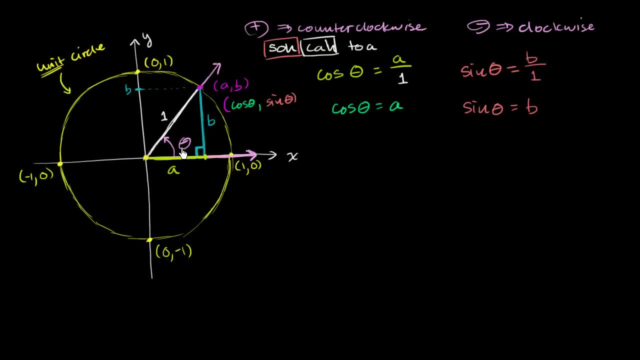 Because SOHCAHTOA has a point. Soh Cah Toa has a problem. It works out fine if our angle is greater than 0 degrees- if we're dealing with degrees- and if it's less than 90 degrees We can always make it part of a right triangle. 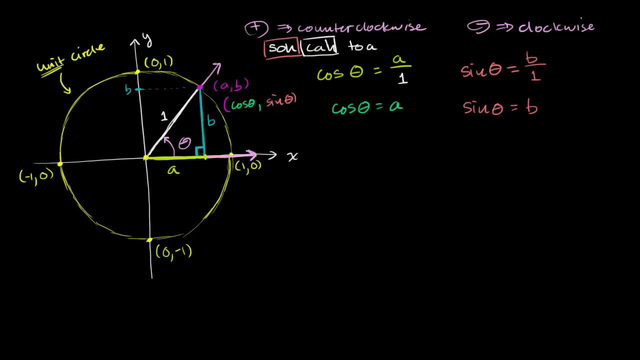 But Soh Cah Toa starts to break down as our angle is either 0, or maybe even becomes negative, or as our angle is 90 degrees or more. You can't have a right triangle with two 90 degree angles in it. 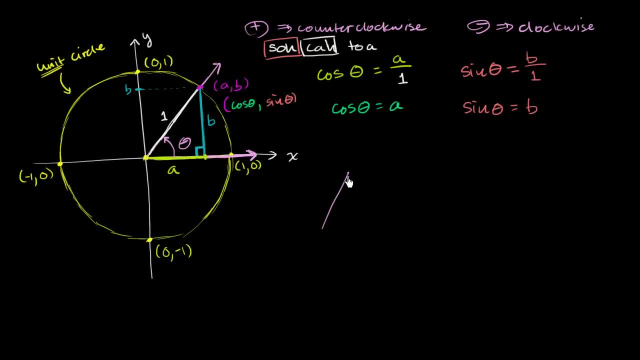 It starts to break down. Let me make this clear. So sure this is a right triangle, so the angle is pretty large. I can make the angle even larger and still have a right triangle even larger, But I can never get quite to 90 degrees.